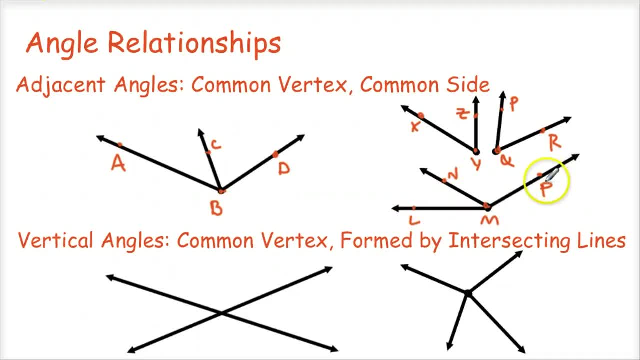 thinking about this big angle, L M P, and then I think about L M N. L M N is actually kind of like inside L M P, So I wouldn't consider that an adjacent angle. So I'd have to be very careful. 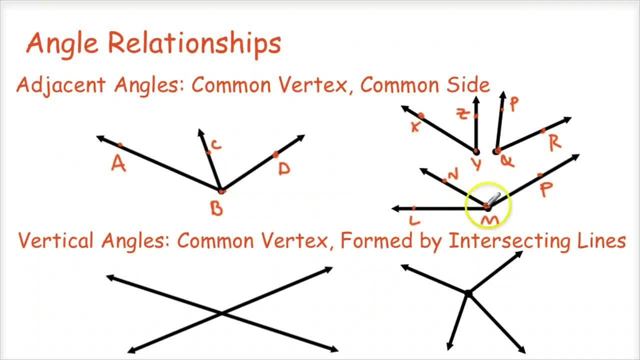 about how I'm reading the question. If it asks me if L M N and L M P are adjacent angles, I would say no. But if it asks me a scenario where it's like A, B C and C, B D, where the common 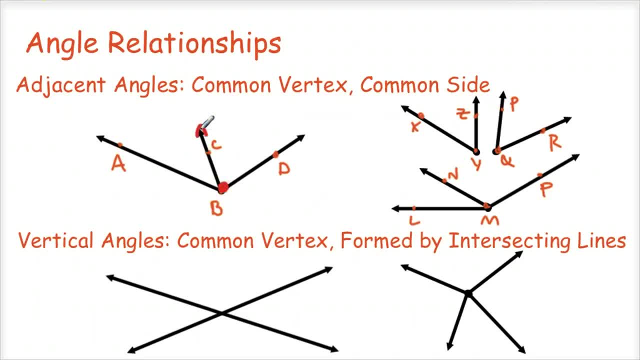 vertex is B and then the common side is C and these two angles are next to each other. so I'm looking at this angle here first and then this angle here second. those would be adjacent. So just be careful about the different scenarios you might see and what exactly is adjacent and what's. 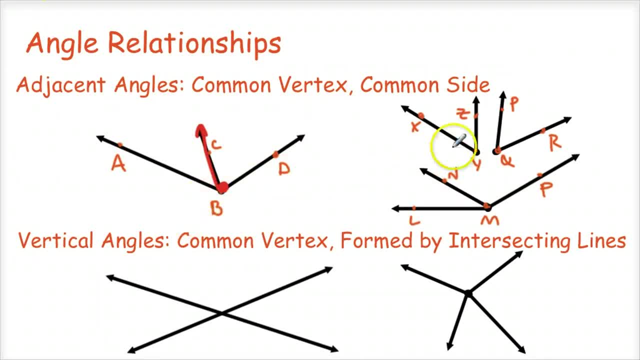 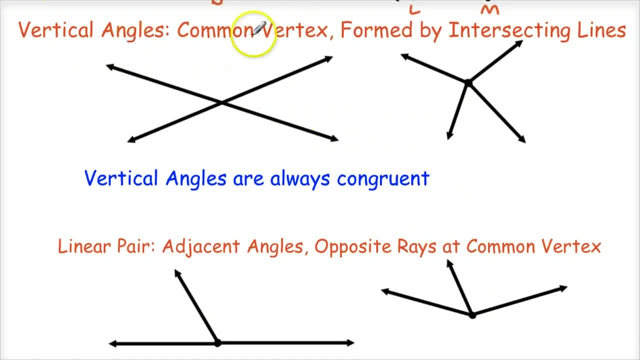 not adjacent. So this one yes, these two no. The next relationship we're going to talk about are vertical angles. So vertical angles again. they have a common vertex: call that X, call this again, we'll call this Y, X, Z and we'll call. 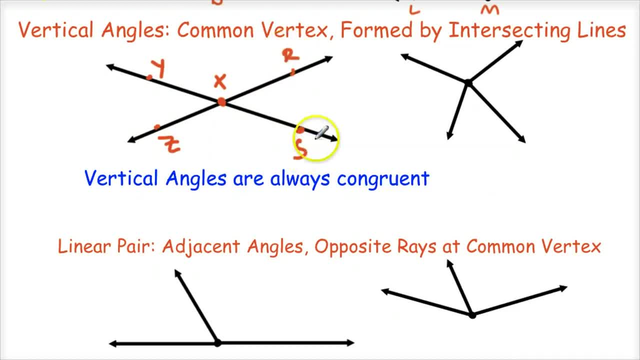 this: R X, S. These two are formed by intersecting lines. So I have Y X, Z and these two are, and Z over here. R X and S. they have a common vertex. they're formed by two intersecting lines. they basically make an X, and so Y X, Z is vertical to, or you. 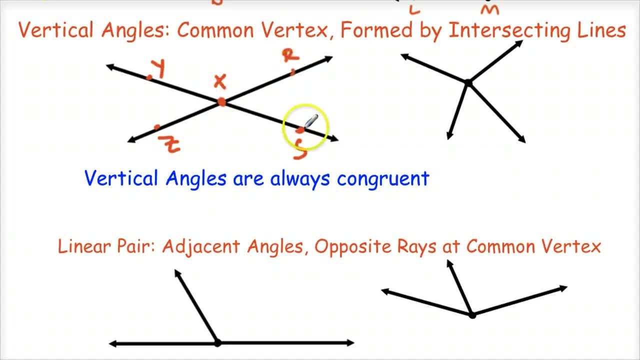 could say vertical width, R X S, so those two are vertical angles. the nice thing about this is the other two angles in this picture are also vertical angles. so Y X R and Z X S are also vertical angles. and another neat fact about vertical angles is that they're always congruent, so angle R X S is congruent. 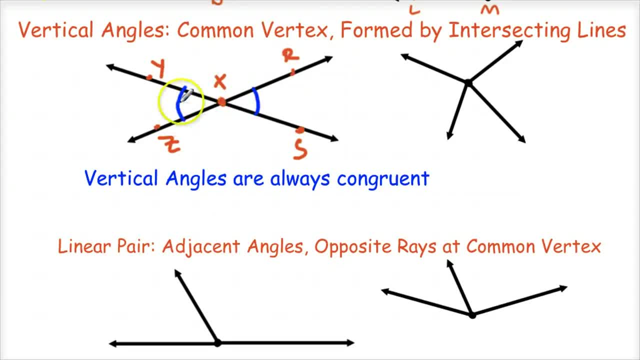 with y x, Z, and so I put the one little arc on those and then remember I said these other two angles in the picture are also congruent. so that means y X R and Z, X R, gute X S are also congruent. They're congruent to each other, but not to these. 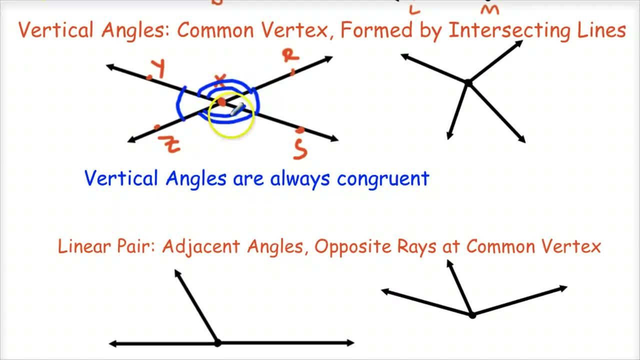 other two. so that's why they get two arcs, to distinguish that those two are congruent as opposed to the one arc on the other one. Okay, so that's what vertical angles look like. Here I have a diagram that kinda looks like an X. 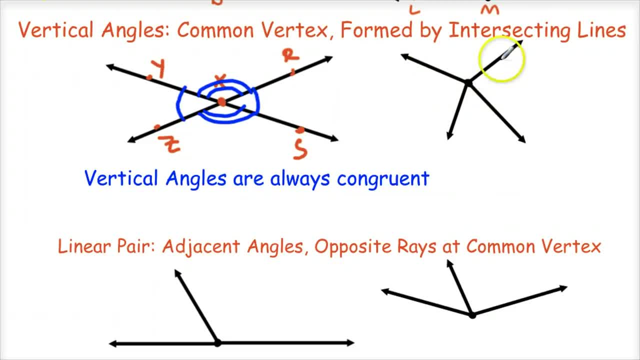 but these are all just four rays that are extending from the same endpoint. These aren't intersecting lines, right? because if I look clearly here, this line does not, or this ray does not line up with this ray, so that's not. 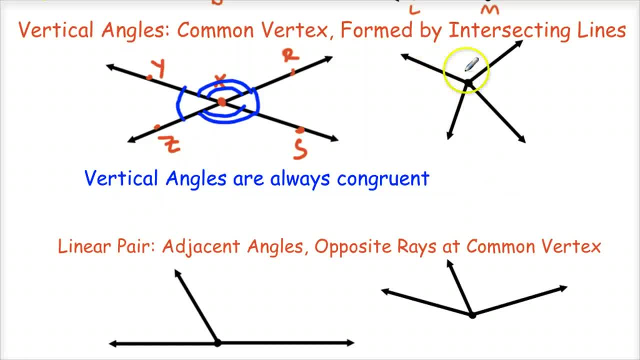 a case of vertical angles. So even though I can see there's angles like across from each other, they're not quite made up by intersecting lines. so this is a scenario where it's not. So you can think of adjacent angles as next two. 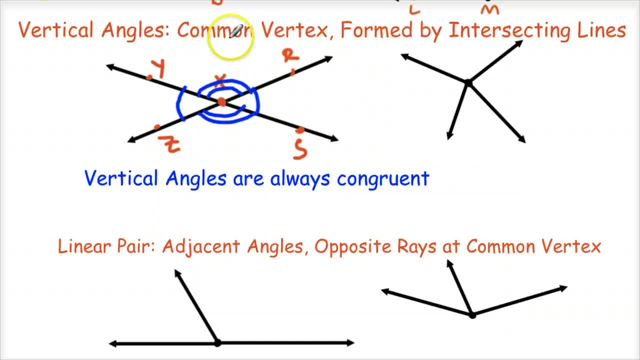 vertical angles as across. but the special thing with vertical angles is that they have to be intersecting lines, so this has to be opposite rays that go across there. The last thing is a linear pair. We'll talk about this. It's an adjacent angle or a set of adjacent angles. 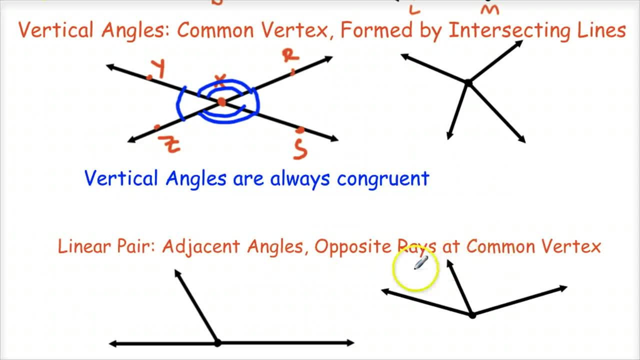 and they have opposite rays at a common vertex. So here again is an example of a yes scenario and a no scenario. With the linear pair we see that the common vertex is the start of two opposite rays. So that makes up a line. so the bottom is a line. so just like, 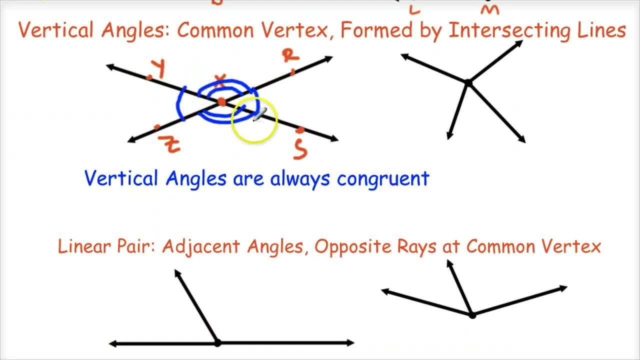 these intersecting lines form a vertical angle. you need a straight line to make a linear pair. So these two angles here we'll just use the numbers to identify these. So we'll call this angle 1, this angle 2, we'll call this angle 3, and this angle 4.. 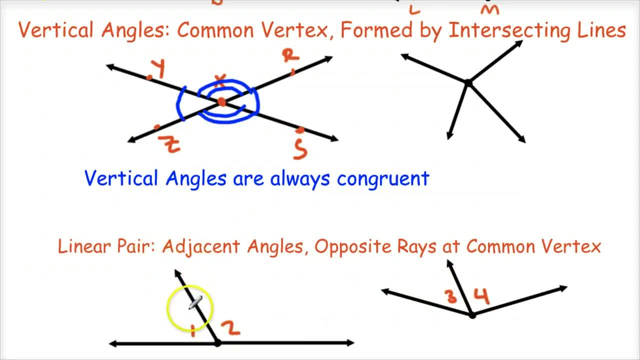 Angle 1 and 2 make up a linear pair because they are adjacent angles, they're next to each other, they share a side and a vertex and they have opposite rays at the vertex. Clearly that's a straight line. 3 and 4 are not a linear pair. 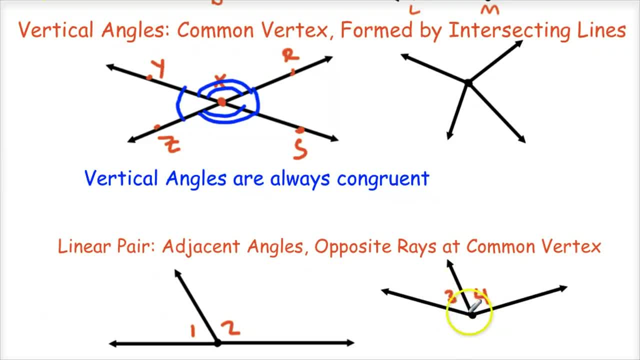 because, even though they're adjacent, they have a common side and a common vertex. at that common vertex, I don't have opposite rays. This doesn't make a line. This ray is going up in this direction. this ray is going up in. 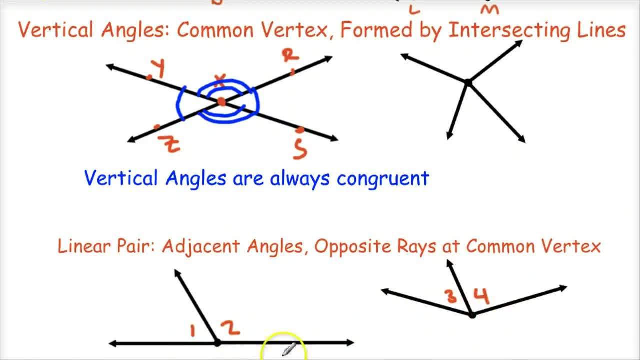 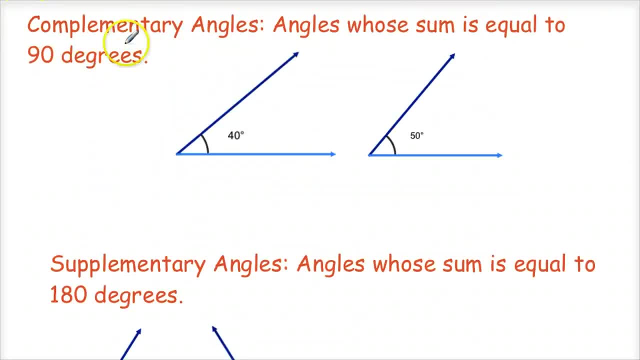 this direction. It's not a straight line across like that is. So those are your three basic relationships. we might talk about. Two other relationships that we can talk about are the two other relationships that we talked about. We talked about a lot are complementary and supplementary angles. 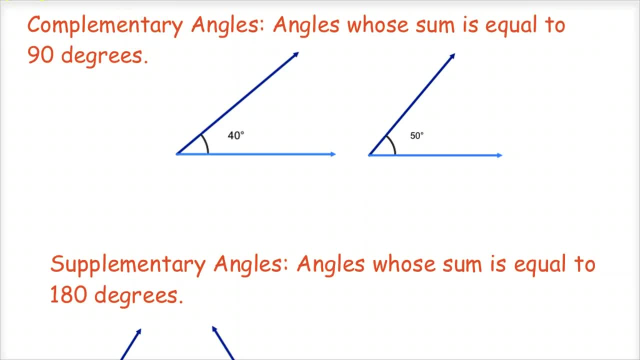 Complementary angles are angles whose sum is equal to 90 degrees. so that means when you add up the measure of two angles, they equal 90 degrees. So here I have two complementary angles. One is 40 degrees, one is 50 degrees. 40 plus 50 equals 90 degrees. 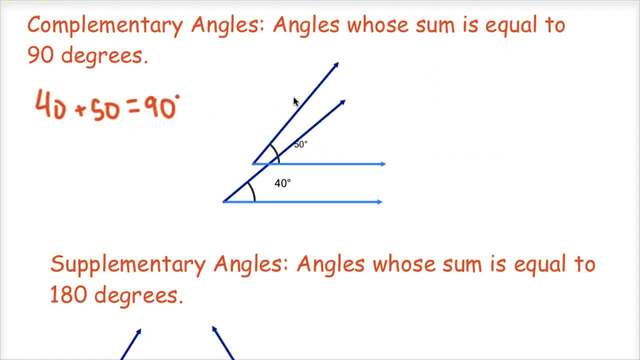 Another way to think about this is: two angles make a right angle. So if I were to put these together and make them adjacent, such that they shared a side and shared a vertex together, that would make a right angle, So that would make 90 degrees. 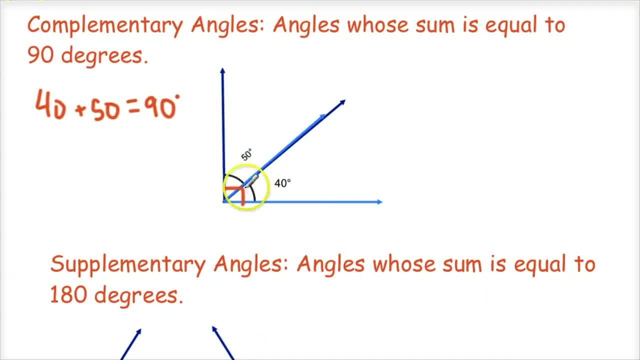 So I would have 50 plus 40 together, that makes 90.. So complementary angles. their sum is 90 and if you were to put them together they would make. if you made them adjacent angles, I should say they would make a right angle. 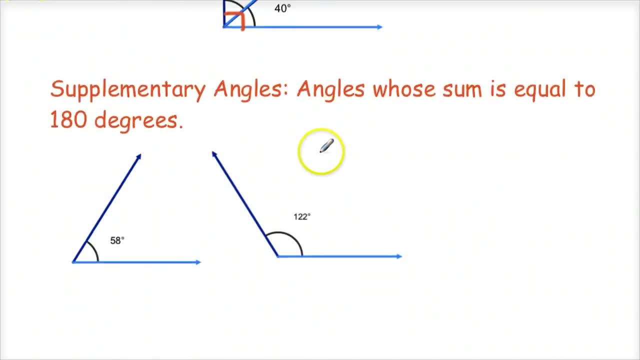 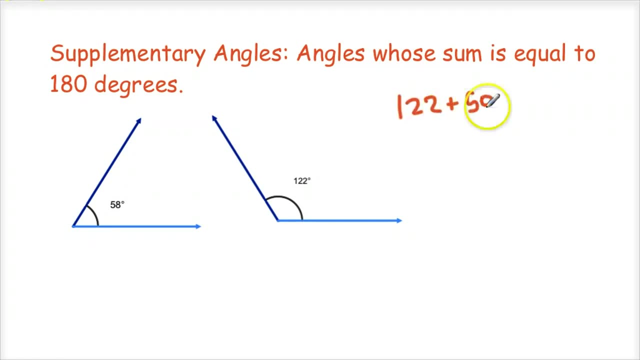 Down here with supplementary angles. those are angles whose sum is equal to 180. So in this case we said 122 degrees plus 58 degrees equals 180 degrees. Okay, so, supplementary 180, complementary 90. And again we can move these angles around. 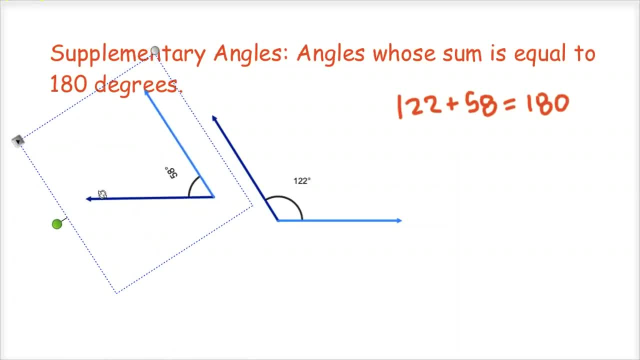 If I made these two adjacent angles and put them next to each other such that they shared a vertex and a common side, they would make up a linear pair Right, so they would make it so that that bottom line is opposite, or opposite raised, and they would add up to be: 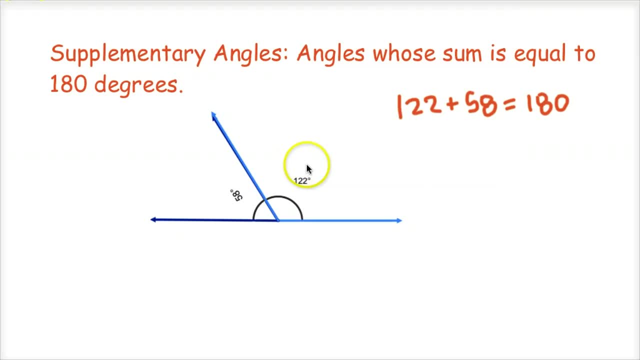 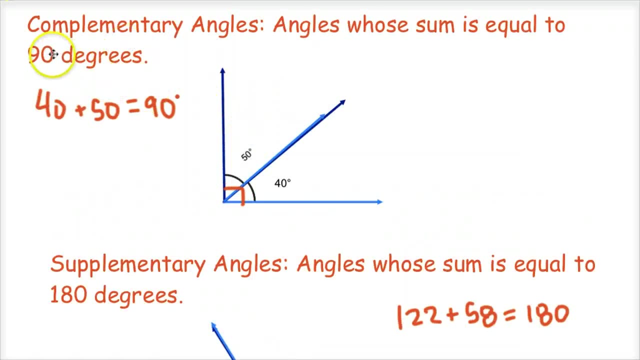 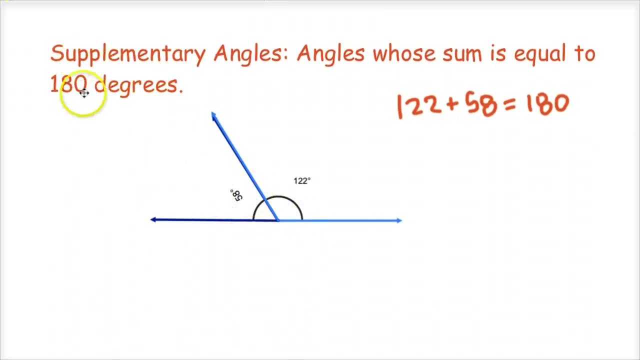 180.. So that's another easy way you can tell from a diagram- is basically, if the two angles, when they're adjacent, make up a right angle, that's means they're complementary 90 degrees. and if they're put together and they make up a linear pair, it means they're supplementary and their sum 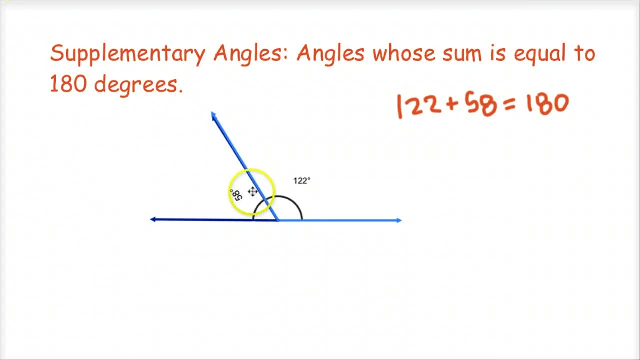 is 180 degrees. Okay, and we'll probably have some examples in class where you'll be using some algebra to finish out like the missing you could. they would say like oh, this angle is 122 degrees and find this is 4x and say that this 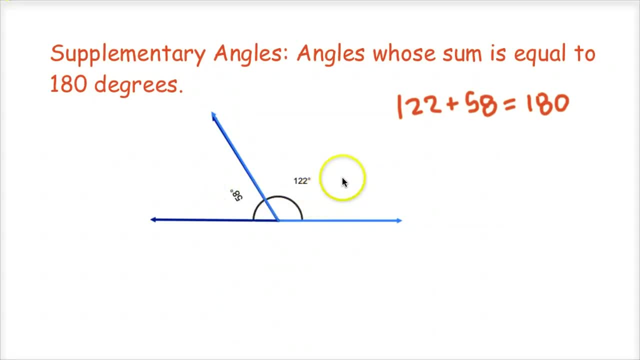 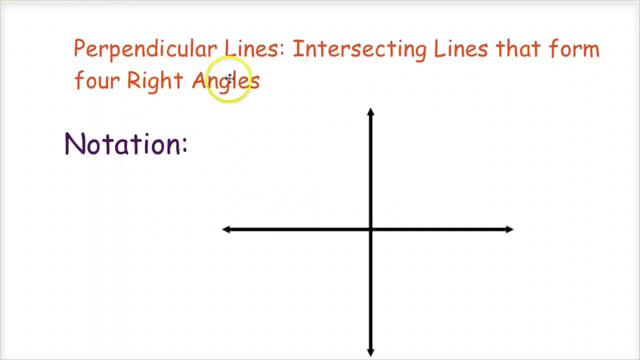 together. they're supplementary, so you'd say 4x plus 122 equals 180 and solve for that. But we'll do that in class, So we don't need to do any examples right now. Last thing we want to talk about are perpendicular lines. 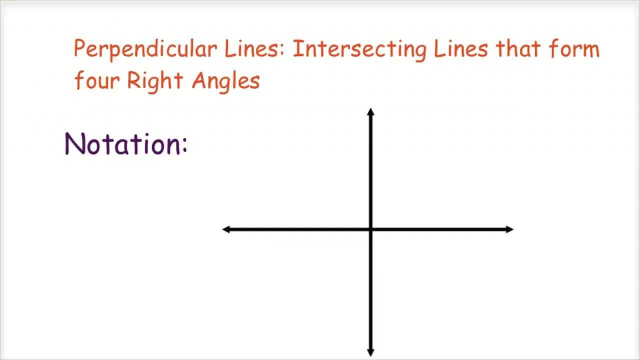 So they are intersecting lines that form four right angles. So if I look at something like this, it's pretty clear. Let's say we have line AB and CD. They are intersecting lines. AB intersects line CD such that they form four right angles. So 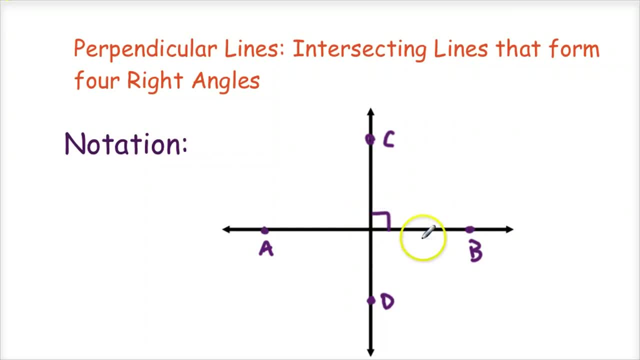 the notation for a right angle is just a little box in the corner. I think we talked about that already. If you look at this, all four of these make right angles. So if we call this point in the middle, we'll call that point P. 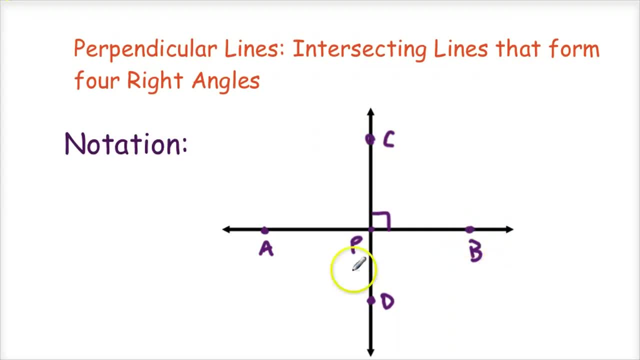 So we can say that angle: CPB is 90 degrees, APB, APC, I should say- is 90 degrees. APD is 90.. DPB is 90.. So these are all 90 degree angles. Um, nice easy. We can do some other examples. 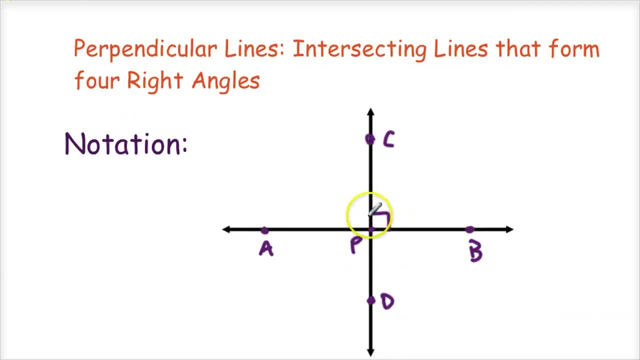 with this, which I'll show you in a second. But just know that these are 90 degrees and that's the definition of perpendicular lines. If you want to use the notation, you would say: line AB is perpendicular to line CD And this is the notation for perpendicular to. It looks like. 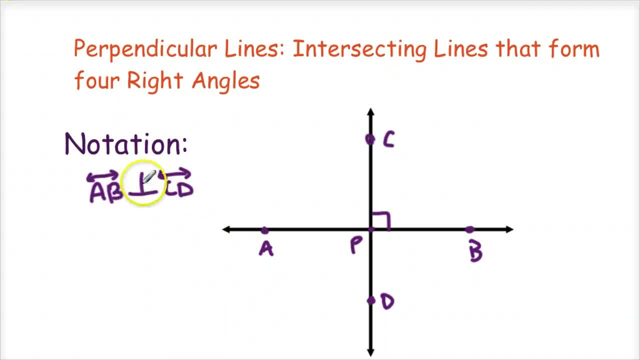 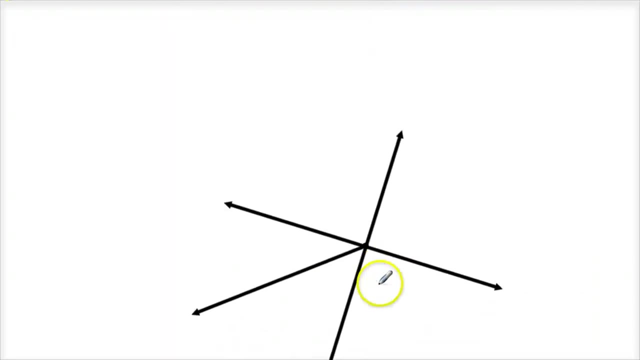 an upside down capital T, So it looks like one line meeting the bottom line at a right angle. So that's how we would distinguish that AB is perpendicular to CD. So that's pretty easy to see when we have it just like in a diagram like that. 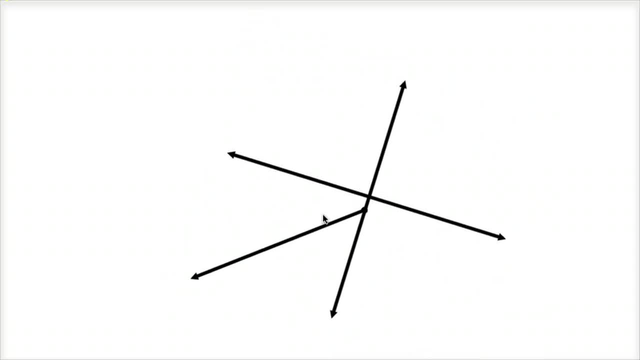 But in this case, down here, let's say we have it where it's not so clear that it's 90 degrees maybe. Uh, we'll just have to be careful about you know, when the diagrams don't look as easy as the way that we see them up top. 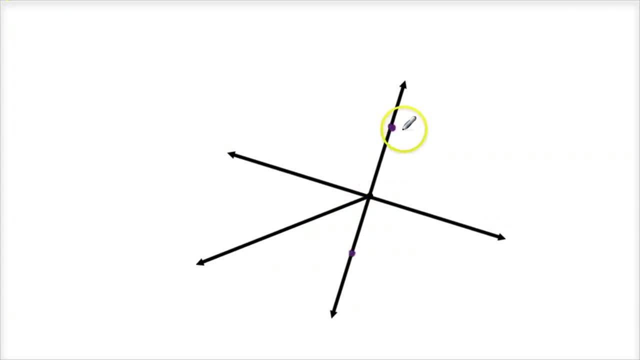 So here again, let's call this DE, call this F, G, and I'll call this H, and then we'll call our vertex there, we'll call that X. Okay, so in this case I could just say: you know, DE is perpendicular to GF, And then you would know that all these four angles are 90 degrees, which is nice, because 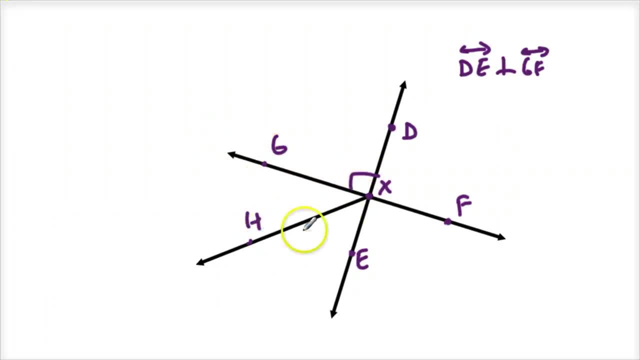 then it tells you something about the relationship between GXH and HXE. So if these two lines are perpendicular and every angle in here is 90 degrees, then that tells me that GH or GXH and HXE then must be complementary, Because those two angles together. 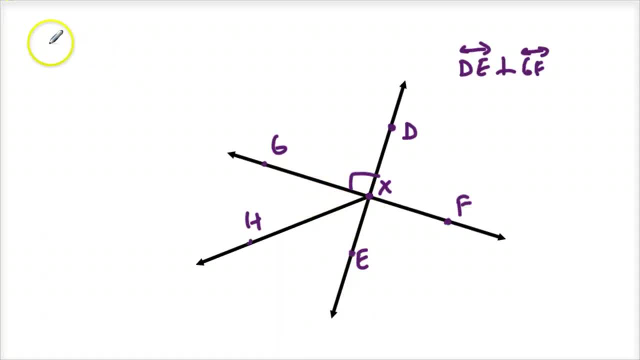 make up a 90 degree angle. So you can say: angle GXH and angle HXE are complementary. And remember, complementary means they add up to 90, their sum equals 90 because those are the two adjacent angles that fill out GXE, which is 90 degrees. 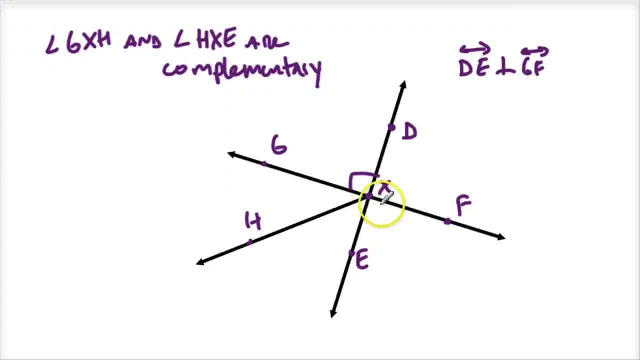 So in this case they're not- which we know is a 90 degree angle, because these two lines are perpendicular. so with this we'll do some other algebra problems. so let's say that angle gx- h is 3x plus 6 degrees, and we'll say hxe. 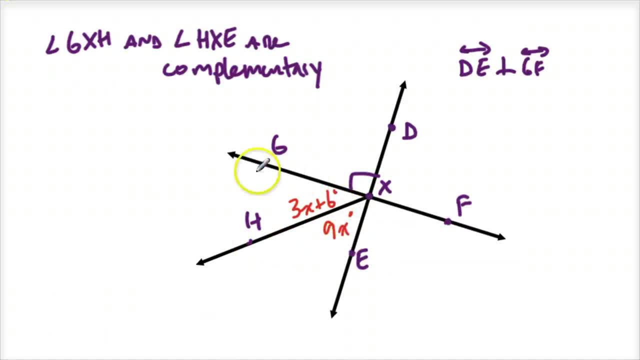 is 9x degrees and we'll say: solve for x or find their angle measure. whatever we want to do with this case, we know that 3x plus 6 plus 9x equals 90 degrees. we know they're complementary because the two of them together make up that right angle. that means they add up to 90. so we